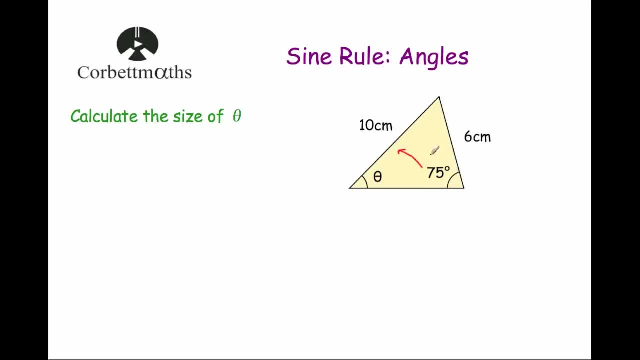 So the tens opposite the 75 degrees and we've got the length of this side being six and that's the side opposite the Vita. So let's plug those in Or let's substitute those into the formula. So the formula is: Sine capital A over a equals Sine capital B over little b. 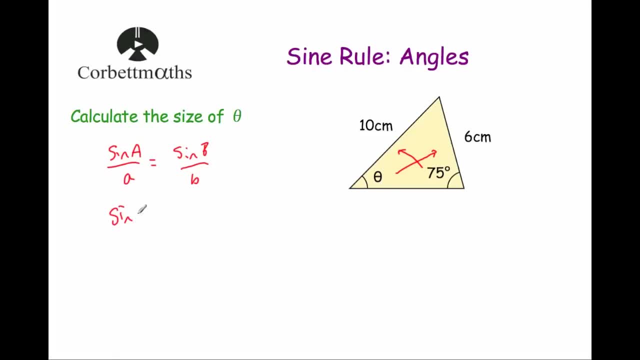 So we've got our Sine Vita. So Sine Vita over the length of the side opposite it, So that's over six, is equal to Sine B, So Sine 75 degrees divided by the length of the side opposite, So divided by 10.. 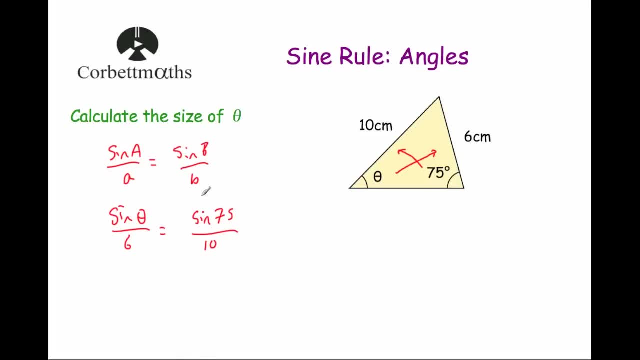 Okay, So we can now work this out. So I'm going to work out my Sine 75 divided by 10.. So it's going to be Sine Vita divided by 6 equals and Sine 75 divided by 10.. 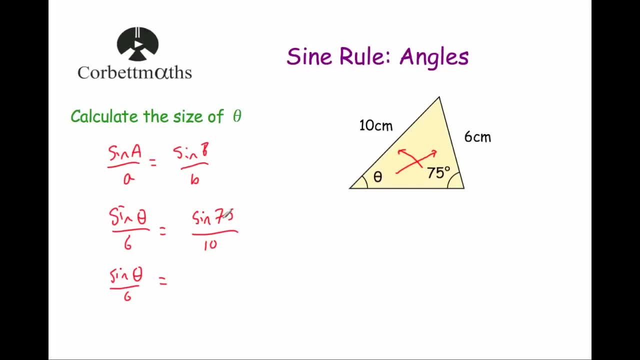 Well, that's going to be equal to Sine 75 divided by 10, and that's equal to 0.0965, and so on. I'm not going to write down the whole display, But what I'm going to do is: I'm not going to write that. 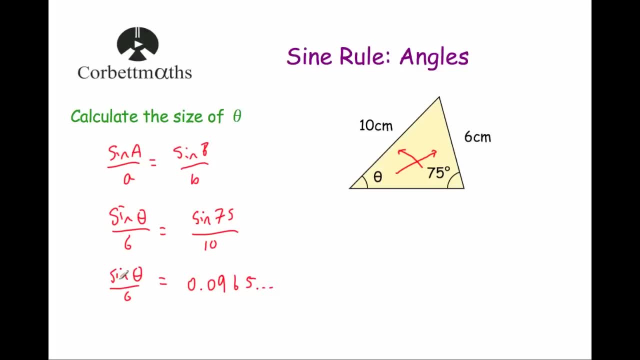 I'm going to keep that on my calculator display. And now I don't want to know what Sine Vita over 10 is. So I'm going to multiply both sides of this equation by 6.. So that's going to give me Sine Vita equals. 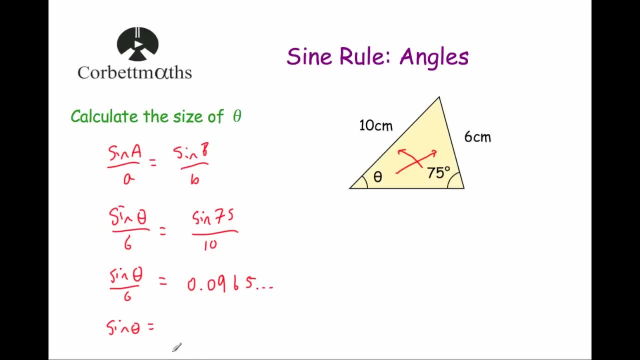 And I'm going to times this by 6.. So multiply by 6 gives me the answer of 0.57955, and so on. Okay, Again, I'm not going to round this Now. in this question I've been asked to work out the size of the angle Vita. 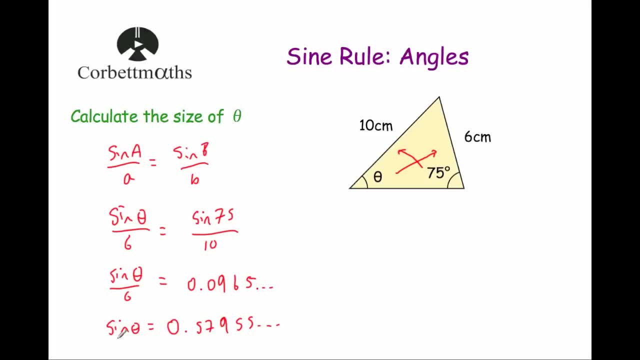 I haven't been asked to work out the size of Sine Vita, So I'm going to want to work out what Vita is. So I'm going to press shift, Press shift Sine or the inverse Sine, So I'm going to do Sine minus 1 of 0.57955 and so on. 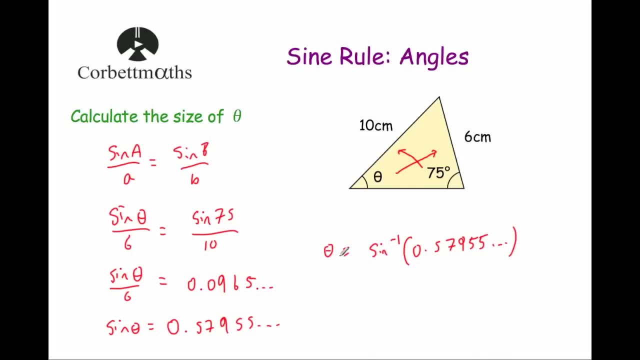 And that will give me the size of the angle Vita. So on my calculator I just press shift Sine And I've already got my answer there. So I'm going to press answer and press equals And that's going to give me that Vita is equal to 35.42 degrees. 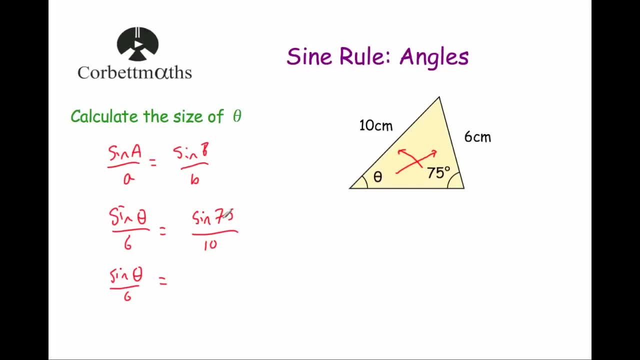 Well, that's going to be equal to sign 75 divided by ten, and that's equal to 0.0965, and so on. I'm not going to write down the whole display, but what I'm going to do is I'm not going to run that. 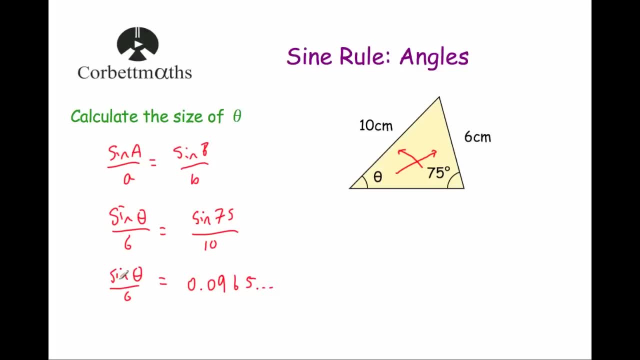 I'm going to keep that on my calculator display. And now I don't want to know what sign Vita over six is. So I'm going to multiply both sides of this equation by six, So that's going to give me sign Vita equals. 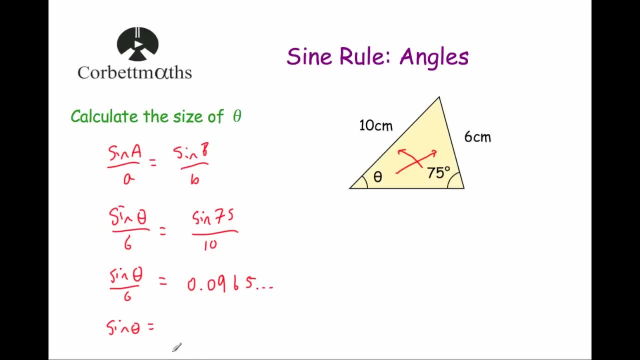 I'm going to times this by six. So multiply by six gives me the answer of 0.57955, and so on. Okay, again, I'm not going to run this Now. in this question I've been asked to work out the size of the angle Vita. 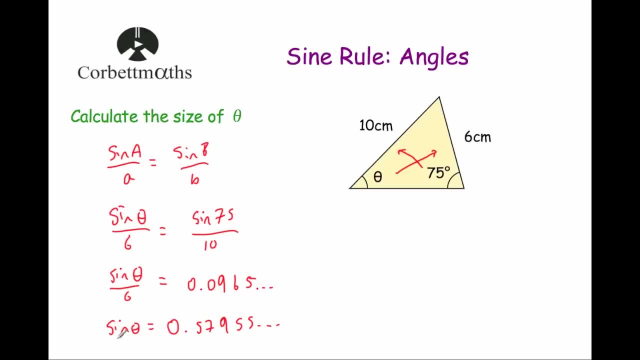 I haven't been asked to work out the size of sign Vita, So I'm going to work. I want to work out what Vita is, So I'm going to press shift sign or the inverse sign, So I'm going to do sign minus one of 0.57955 and so on. 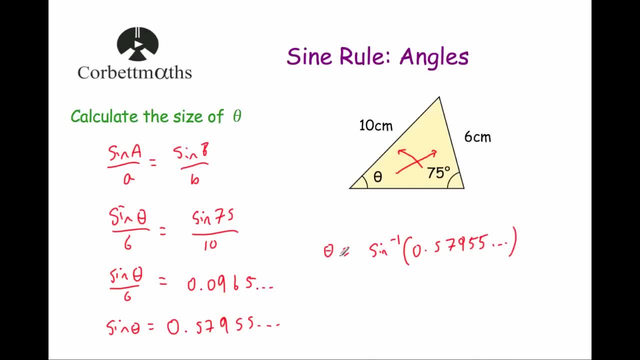 And that will give me the size of the angle Vita. So on my calculator I just press shift sign and I've already got my answer there. So I'm going to press answer and press equals And that's going to give me that Vita is equal to 35.42 degrees and that's the two decimal places. 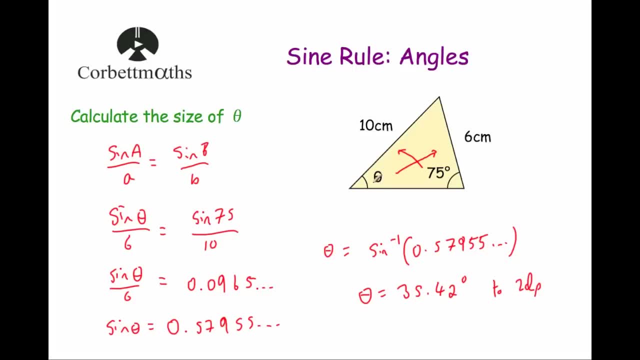 That's it. So the size of this angle Vita is 35.42 degrees. Okay, let's have a look at another example now. Okay, so our next question says: calculate the size of angle BAC. So here we've got this triangle. 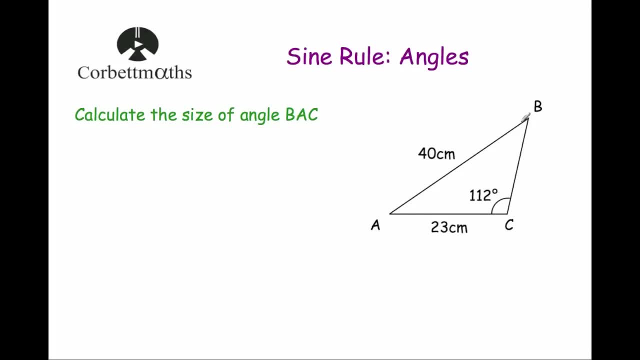 We've got ABC, So we want to find the size of angle BAC. So that's this angle here, Vita. Now, interestingly, in this question, I don't know the length of the side opposite it And you can only use the sign rule if you know the angle and the sides opposite it. 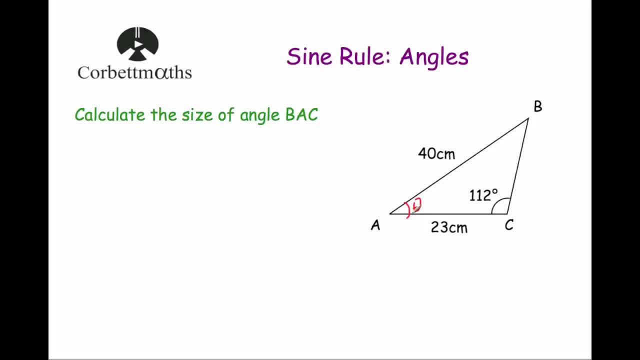 So what I'm actually going to do in this question is, rather than get the size of Vita, I'm going to work at the angle A ABC. I'm going to find what angle ABC is, So I'm going to call this angle up here. 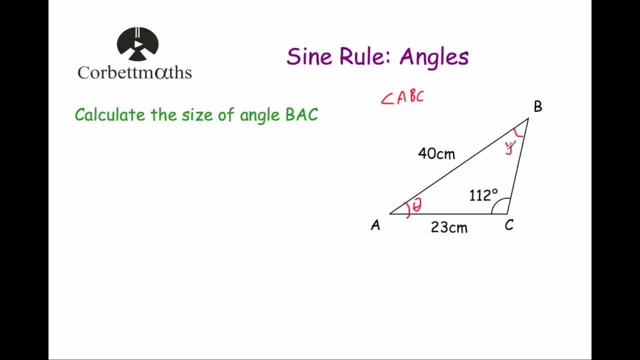 Let's just call it Y. So what I'm going to do is I'm going to find the size of angle Y and then I'll use this angle 112.. And then I'll take those away from 180 and I work at the size of Vita. 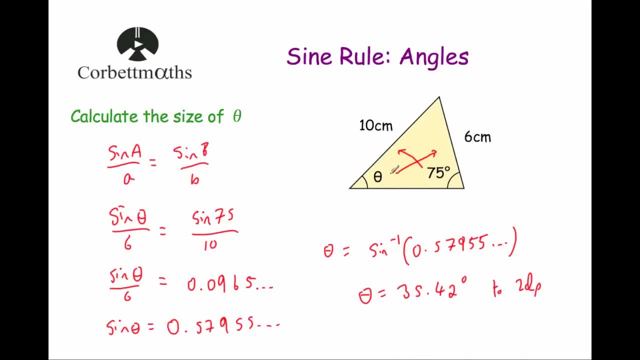 And that's the two decimal places. That's it. So the size of this angle Vita is 35.42.. Okay, Let's have a look at another example now. Okay, So our next question says: calculate the size of angle BAC. 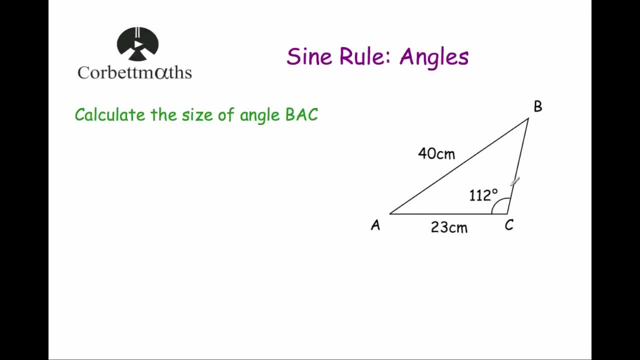 So here we've got this triangle, We've got ABC, So we want to find the size of angle BAC. So that's this angle here, Vita. Now, interestingly in this question, I don't know the length of the side opposite it. 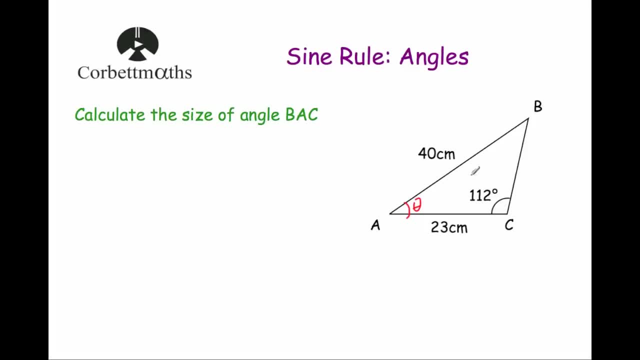 And you can only use the sine rule if you know the angle and the sides opposite it. So what I'm actually going to do in this question is, rather than get the size of Vita, I'm going to work at the angle ABC. I'm going to find what angle ABC is. 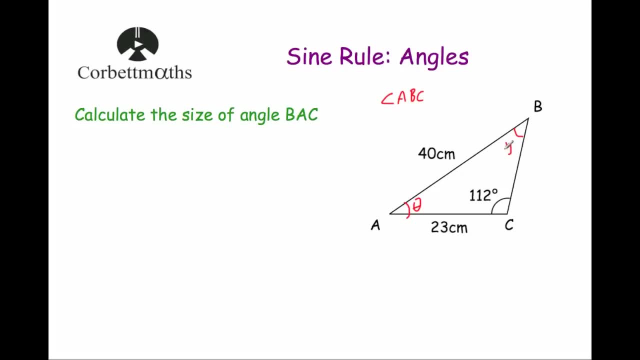 So I'm going to call this angle up here, Let's just call it Y. So what I'm going to do is I'm going to find the size of angle Y And then I'll use this angle 112.. And then I'll take those away from 180 and I'll work out the size of Vita. 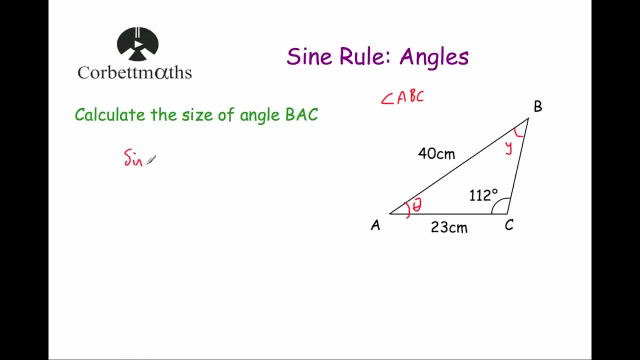 So let's write down what the sine rule is. So the sine rule is: sine A over little a equals sine B over little b. So that's the angle and the side opposite it, the angle and the side opposite it. So we're going to be focusing on the Y. 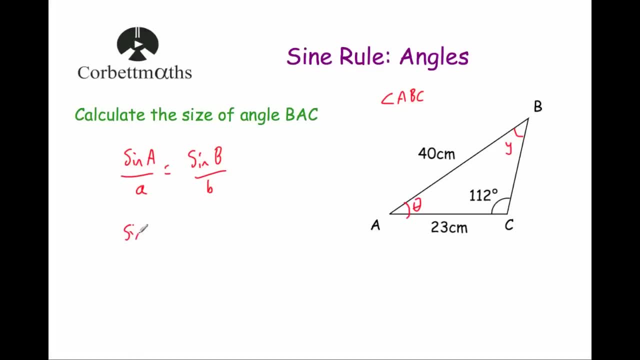 So we want to find what that is. So we're going to write sine Y over, And then it's the side opposite it, So that's over 23 equals, And then we know the 40 centimeters and the 112 degrees. 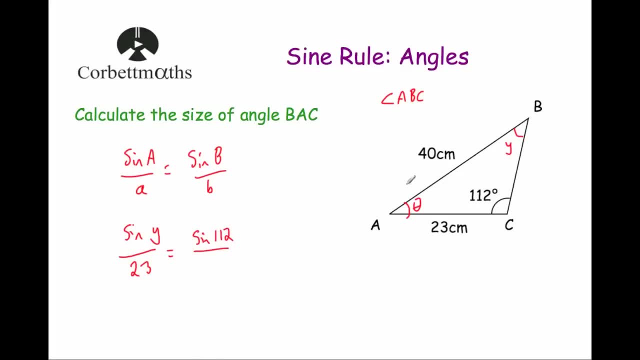 So we're going to use sine 112 over 40. And again we're going to work out what this is in the calculator. So we're going to do sine 112, close brackets divided by 40. And that's equal to sine Y over 23.. 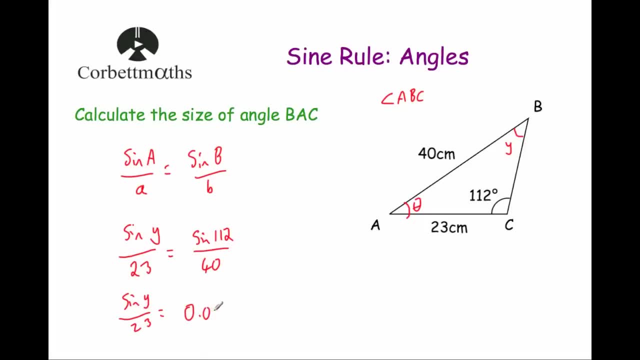 And that's equal to 0.023179 and so on. But I don't want to know what that is divided by 23.. So I'm going to multiply both sides of this equation by 23.. So that could be sine Y equals. 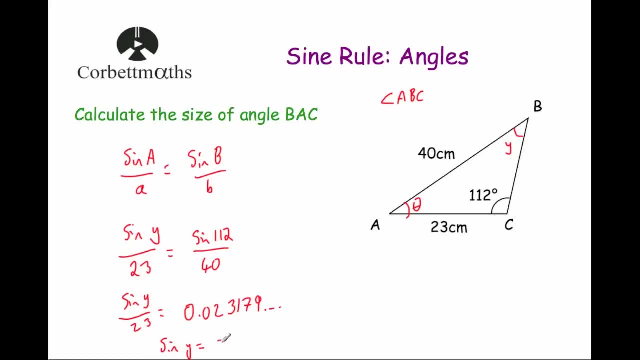 Timesing by 23, is equal to 0.53313. so on Again, don't round any of these numbers. And I don't want to know what the sine of Y is. I want to know what Y is. So Y equals the inverse sine or shift sine. 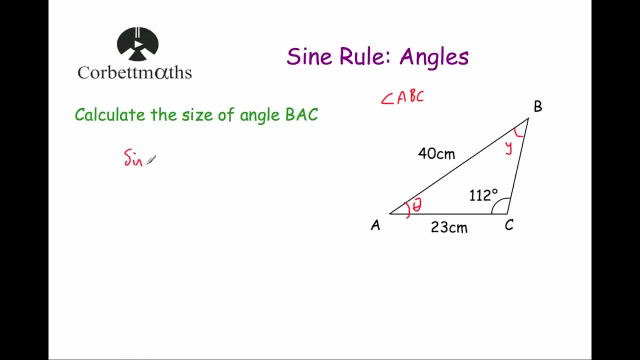 So let's write down what the sign rule is. So the sign rule is: sine A over little a equals sine B over little b. So that's the angle and the side opposite it, the angle and the side opposite it. So we're going to be focusing on 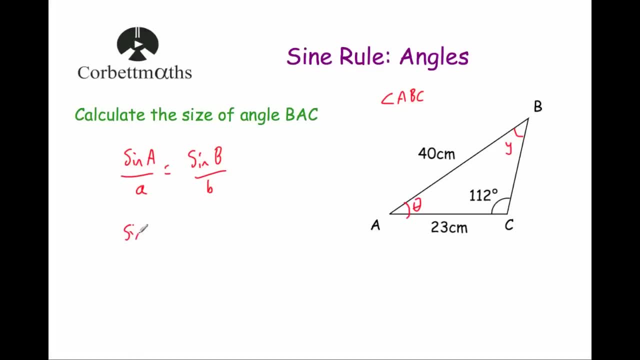 The Y. So we want to find what that is. So we're going to write sine Y over, and then it's the side opposite it, So that's over 23 equals, And then we know the 40 centimeters and 112 degrees. 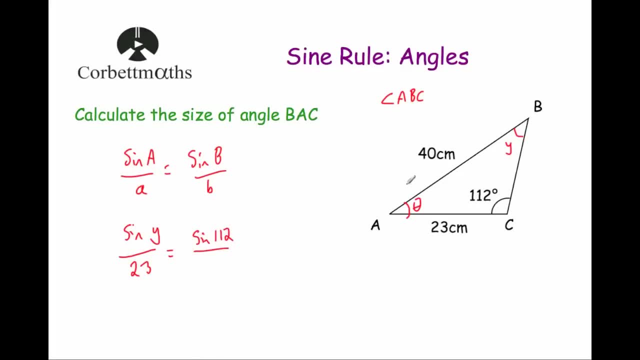 So we're going to use sine 112 over 40. And again we're going to work out what this is in the calculator. So we're going to do sine 112, close brackets divided by 40. And that's equal to sine Y over 23.. 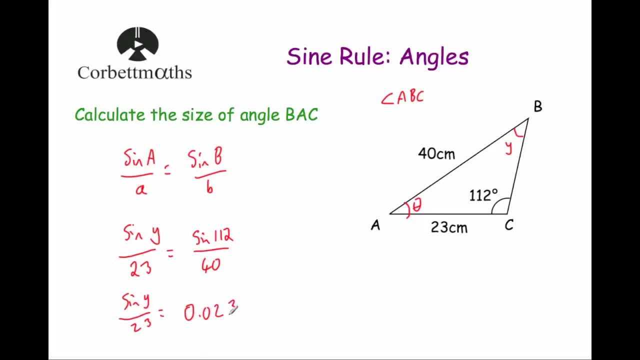 And that's equal to 0.023179, and so on. But I don't want to know what that is divided by 23.. So I'm going to multiply both sides of this equation by 23.. So that could be: sine Y, equals times by 23 is equal to 0.53313, so on. 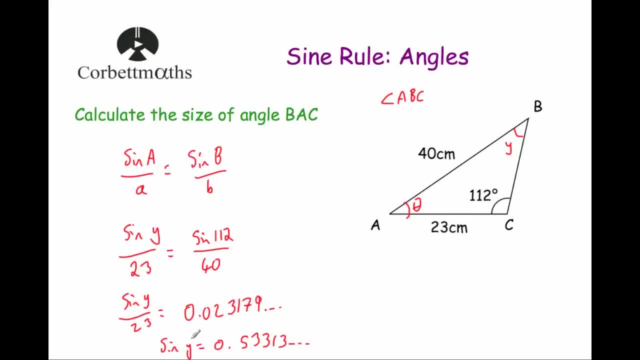 Again, don't round any of these numbers And I don't want to know what the sign of Y is. I want to know what Y is. So Y equals the inverse sine or shift sine of 0.5331, and so on. 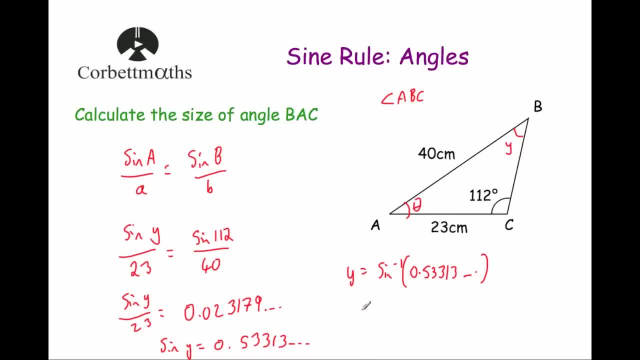 And that gives us, when we press shift, sine and answer, That gives us that Y is equal to 32.217, so on degrees. But we don't want to know what Y is. But let's actually label it there: 32.217, so on. 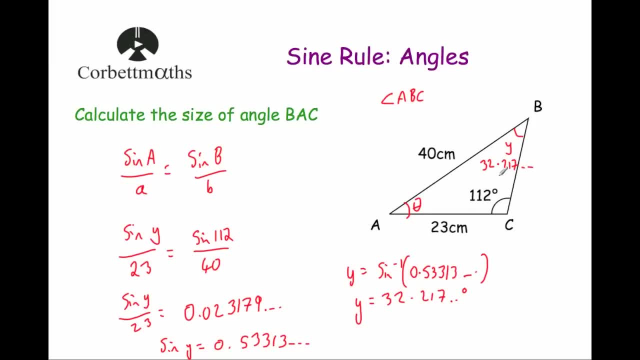 We want to find the size of the angle Vita, The angle BA. So we're going to add these two angles together And we're going to take it away from 180.. So 180 minus the sum of 32.217, so on plus 112.. 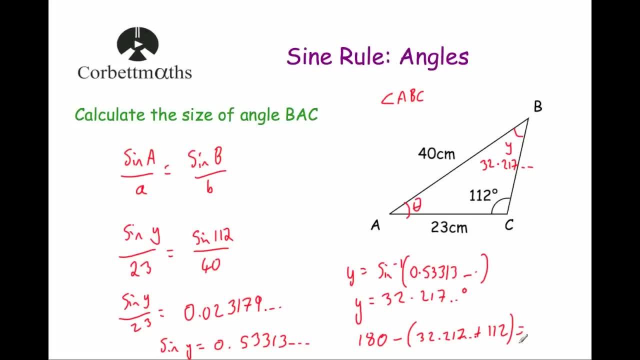 And that gives us: So let's add 112 to that number, Let's take it away from 180.. And that gives us the angle BAC. So this angle here, Vita, is equal to 35.8 degrees, to one decimal place.